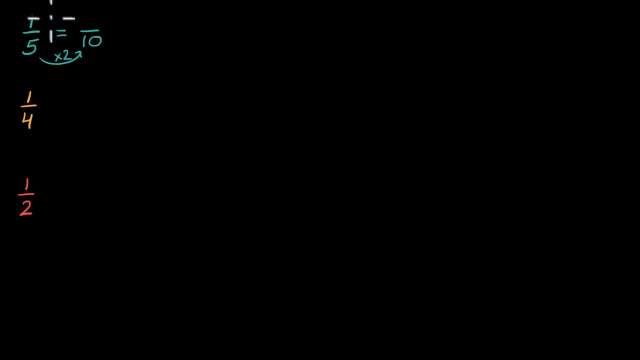 you have to multiply the denominator by two. So let's multiply the numerator by two as well. So 1 5th one times two is the same thing as two tenths, And we know how to represent that. in decimal notation That's going to be 0.2. 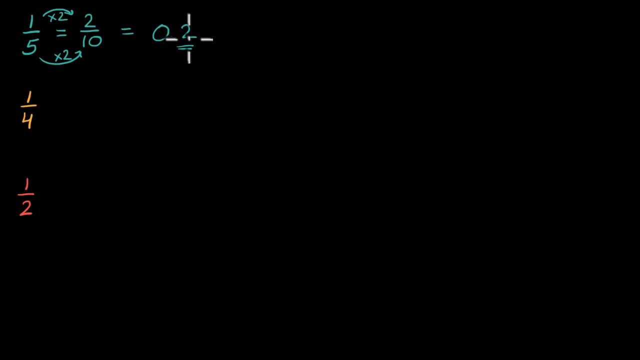 This is the tenths place, So we have exactly two tenths. Now let's do 1, 4th. Same idea. How can I represent this as a decimal? Well, at first you might say: well, can I represent this as a certain number of tenths? 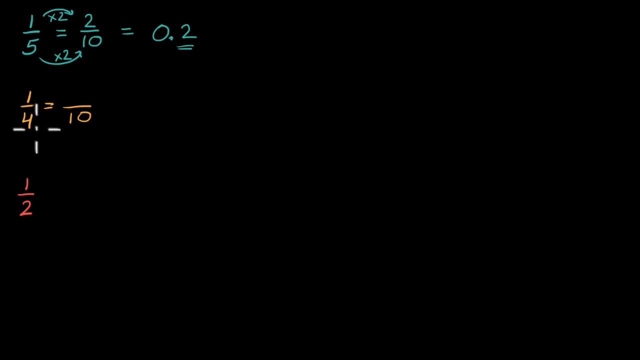 But- and you could do it this way- but 10 isn't a multiple of four. So let's see if we can do it in terms of hundredths, because hundred is a multiple of four. Well, to go from four to a hundred, 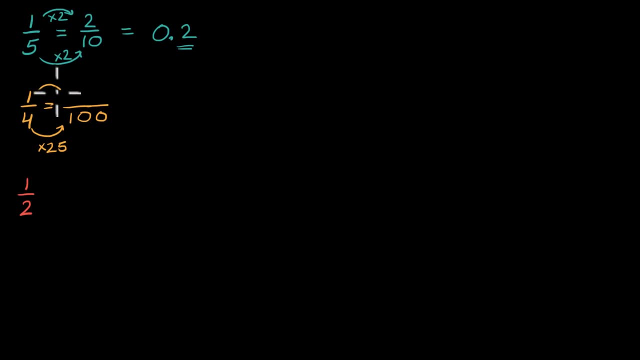 you have to multiply by 25.. So let's multiply the numerator by 25 to get an equivalent fraction. So one times 25 is 25.. So 1: 4th is equal to 25 hundredths, And we can represent that in decimal notation as 25 hundredths. 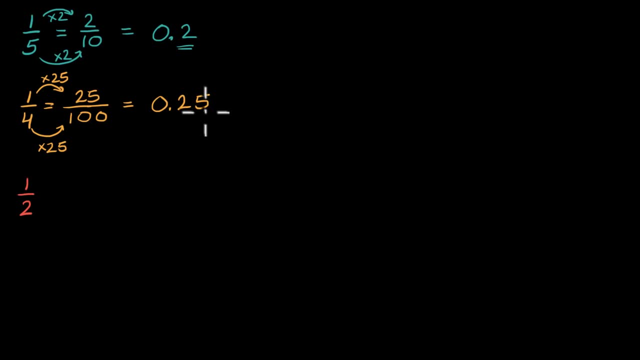 which we could also consider two tenths and 500.. Now let's do 1: half, Same exact idea. Well, 10 is a multiple of two, So we can think about this in terms of tenths. So, to go from two to 10, we multiply by five. 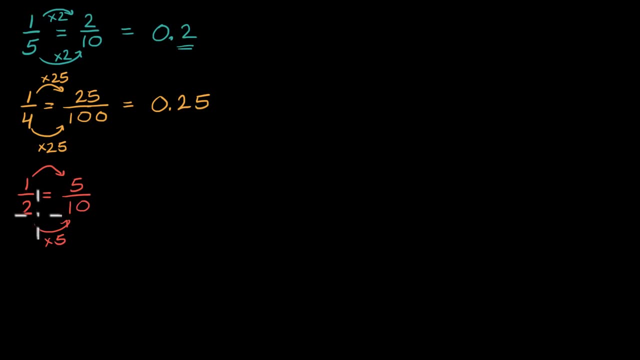 So let's multiply the numerator by five as well. So 1 half is equal to five tenths, which, if you want to represent it as a decimal, is 0.5.. Five tenths, Now. why is this useful? Well, one, you're going to see these fractions. 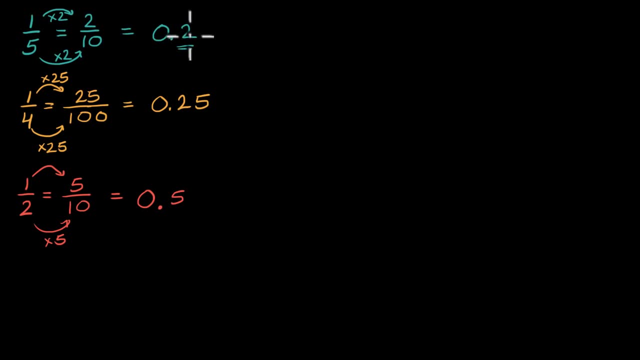 show up a lot in life And you're going to go both ways. If you see two tenths or 20 hundredths to be able to immediately recognize, hey, that's 1, 5th or 25 hundredths. Hey, that's 1 4th or 1 4th. 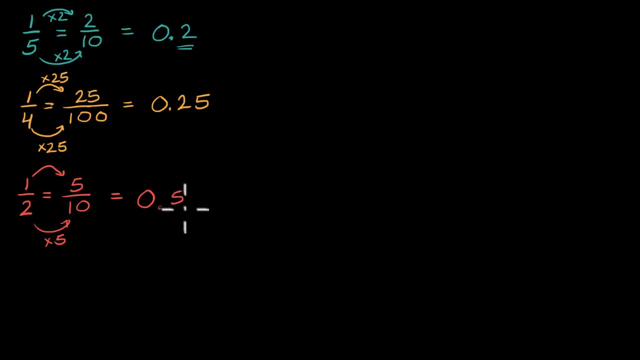 That's 25 hundredths. 1 half is 0.5 or 0.5 is 1 half, And it's not just useful for these three fractions, It's useful for things that are multiple of these three fractions. For example, if someone said: 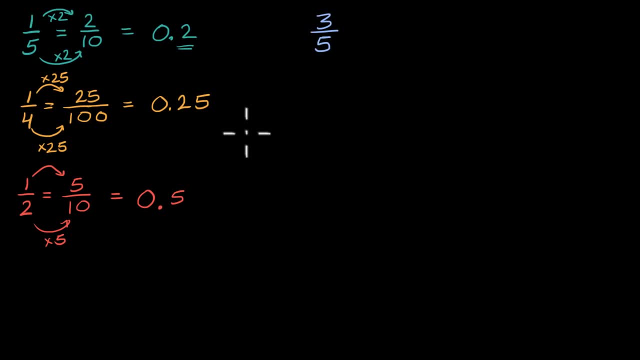 quick. what is 3, 5ths, represented as a decimal? Well, in your brain you could say: well, 3, 5ths, that's just going to be 3 times 1, 5th, And I know that 1, 5th is 2 tenths. 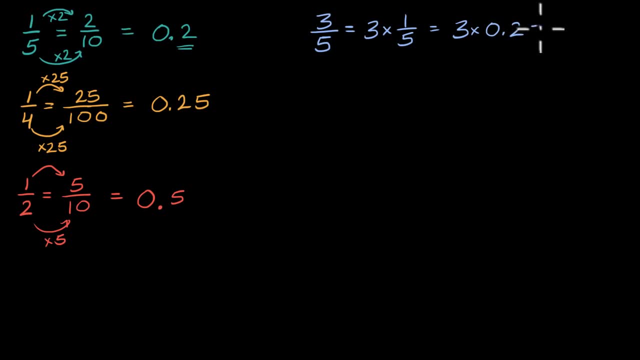 So that's going to be 3 times 2 tenths, which is well, 3 times 2 is 6.. So 3 times 2 tenths is 6 tenths. So really quick you're able to say. 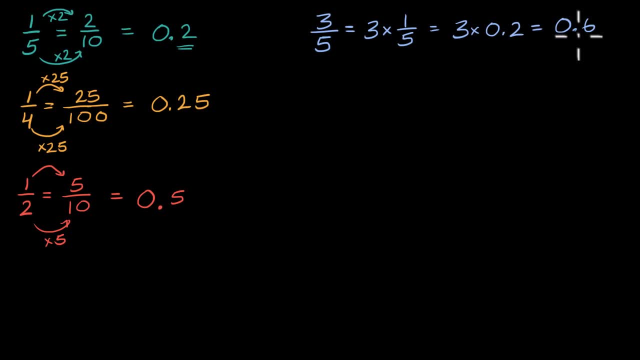 hey, that's 3 5ths is 6 tenths. And you could have gone the other way around. You could have said: 6 tenths is equal to 2 times is equal to 3 times 2 tenths. 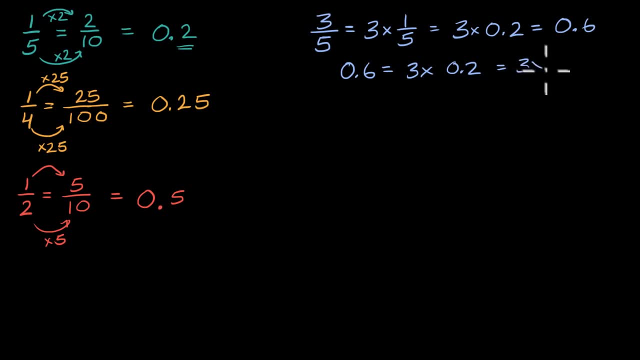 And 2 tenths. you know is 1- 5th, So this is going to be equal to 3 times 1: 5th And, once again, these are just things that you'll get comfortable with the more that you get practice. 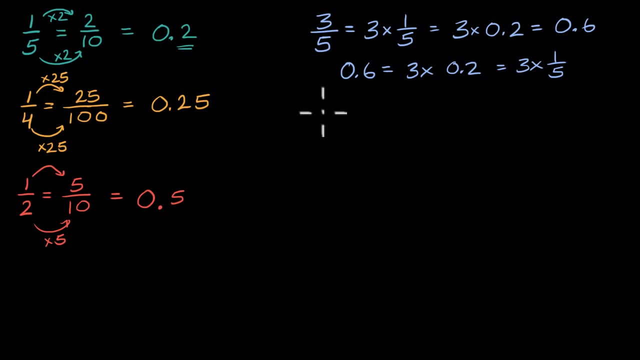 Let's do another one. Let's say you wanted to represent. let's say you wanted to represent. so let me do it another way. 0.75 as a fraction. Pause the video. try to do it yourself. Well, you might immediately recognize. 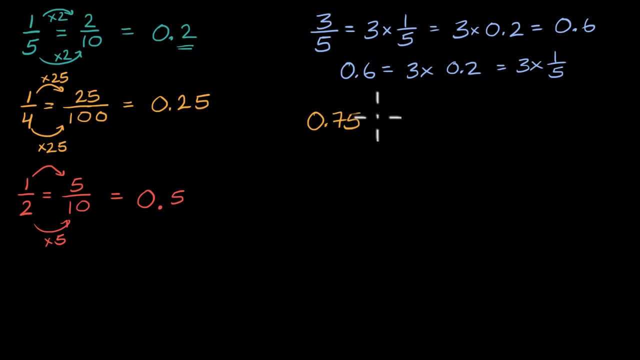 that 0.75 is 3 times 2 5ths. So 0.75 is equal to 3 times 2 5th, And 2- 5th, we already know, is 1- 4th. So this is equal to 3 times 1 4th. 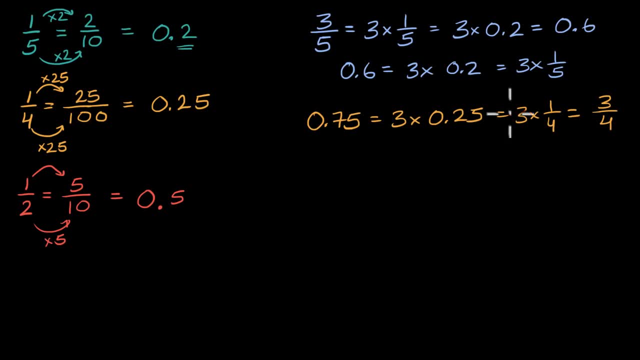 which is equal to 3 4ths, And over time you won't have to do all of this. in your head You'll just recognize 0.75, that's 3 4ths, because 2 5th is 1 4th. 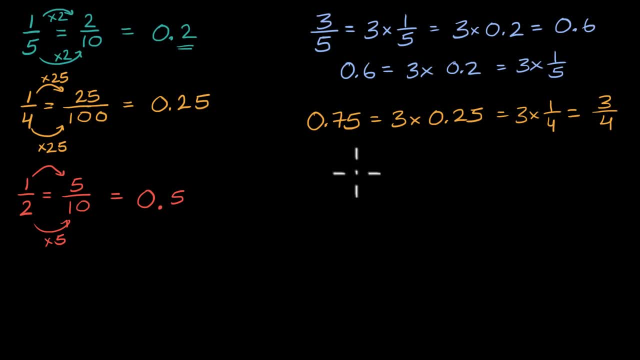 And now let's do, let's say we have, let's say we have 2.5.. And we want to represent that as a fraction. Well, there's a bunch of ways that you could do this. You could say: well, this is 5 times 0.5.. 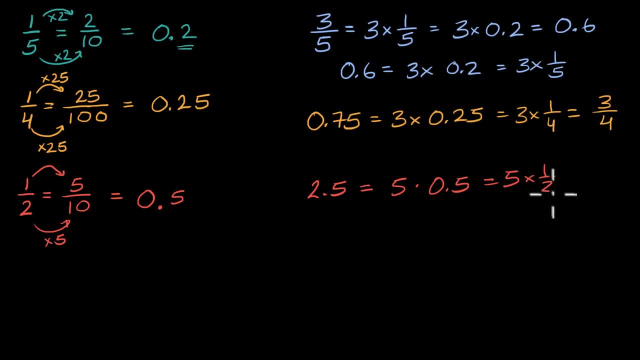 And that's going to be 5 times 1 half. Well, that's going to be 5 halves. It's an improper fraction, but it's a fraction, And so, once again, the whole point here, and you might already be familiar. 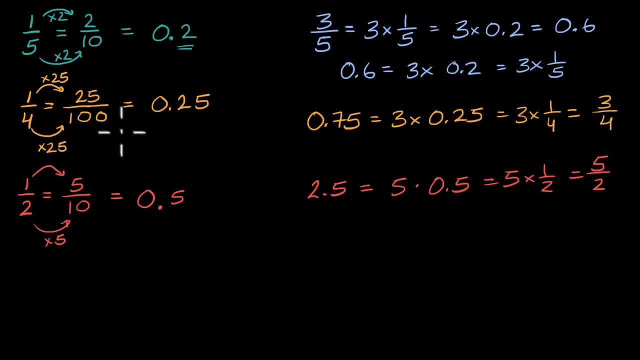 with different ways of converting between fractions and decimals, But if you recognize 1, 5th, 1 4th, 1 half, it's going to be a lot easier. Notice, if you did it the other way around, it would be a little bit more work. 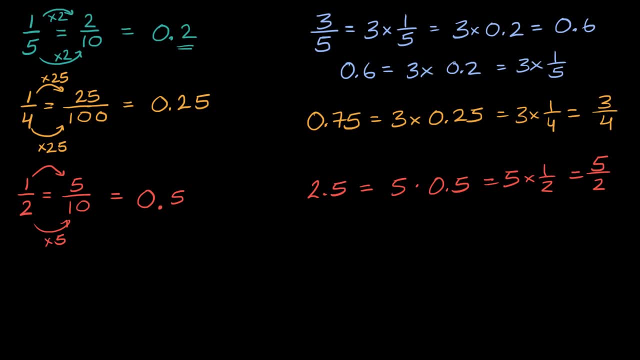 If I said: let me convert 3 5ths to a decimal, well then you would have to divide 5 into 3.. 5 into 3, and you'd say: okay, 5 goes into 3, 0 times. 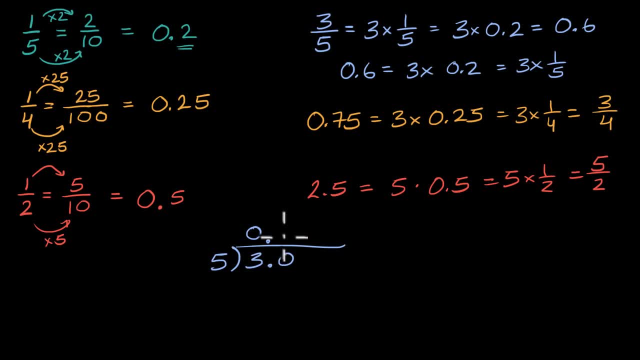 So let's put a decimal here. Now let's go to 30.. 5 goes into 30. 6 times 6 times 5 is 30. You subtract and then you get no remainder. So this wasn't a ton of work. 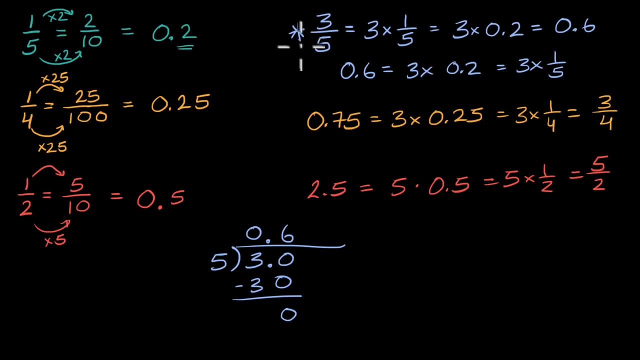 But this one the reason why I like this one: not only is it faster, but it gives you a better intuition for what actually is going on. 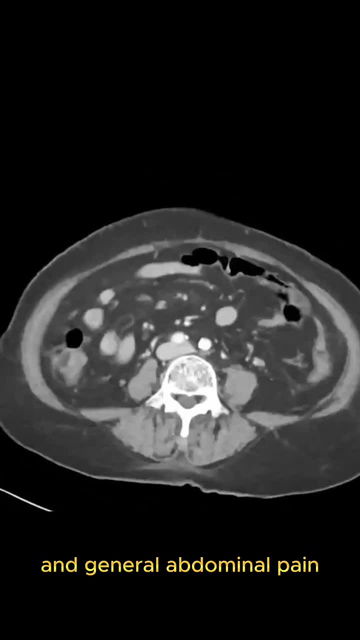 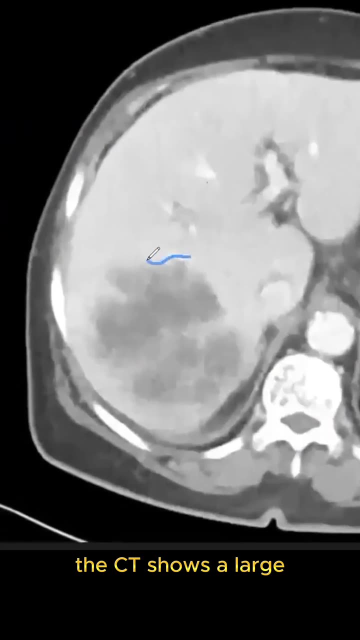 80-year-old male presents with fever, rigors, sweats and generalist abdominal pain, A CT scan is performed. Which of the following do you think is a diagnosis? The CT shows a large clustered hypotense liver mass in the right liver lobe. 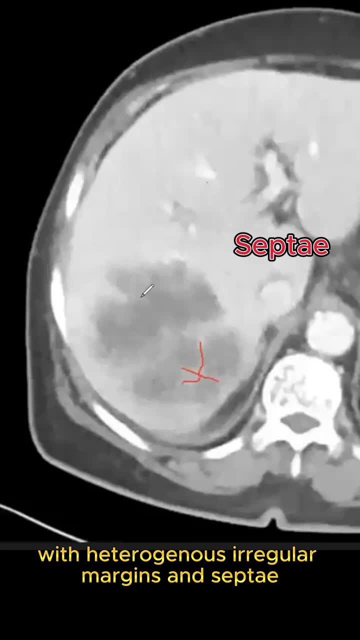 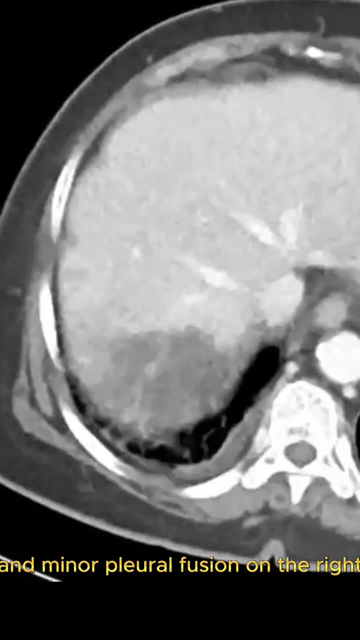 with heterogeneous irregular margins and septae. A tiny gas local is seen within the lesion, along with basal atelectasis and minor pleural fusion on the right. While metastatic liver lesion can present with low density liver mass, it is usually not clustered and it is not